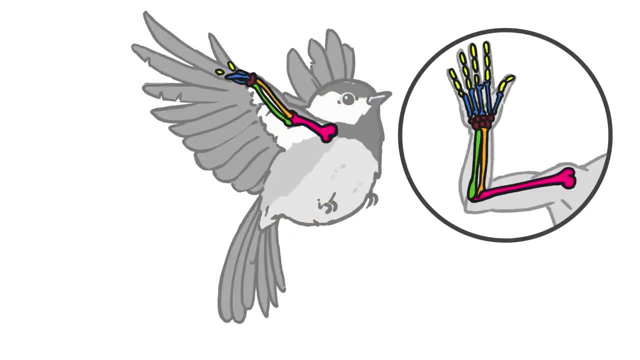 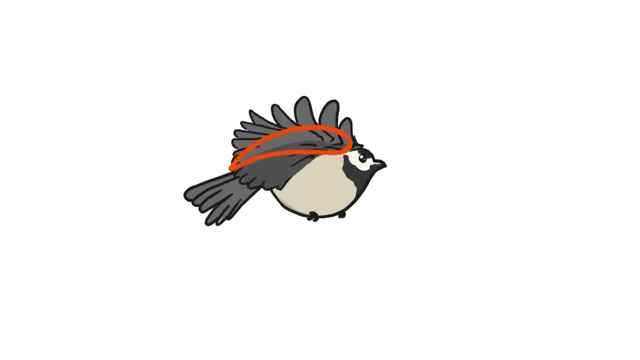 Birds would never get off the ground without their wings. Bird wings are basically modified arms geared toward flying. This is what a bird wing looks like from the side. See how it's curved. When this shape moves through the air, that curve catches the air and redirects it downward. 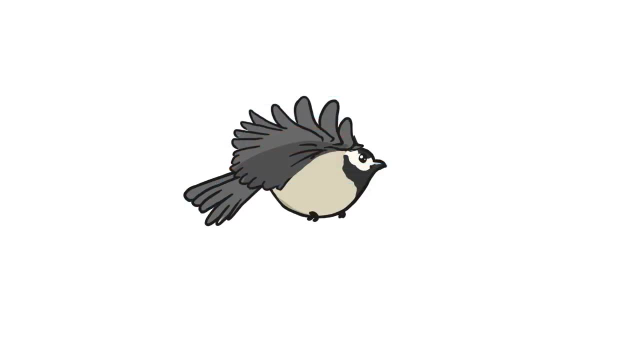 creating a force called lift- To keep the wing moving through the air, the bird has to flap it- generating a force called thrust. As long as enough air is moving across the bird's wing, that wing will soar. But flap as much as they like, birds would not get very far without feathers. 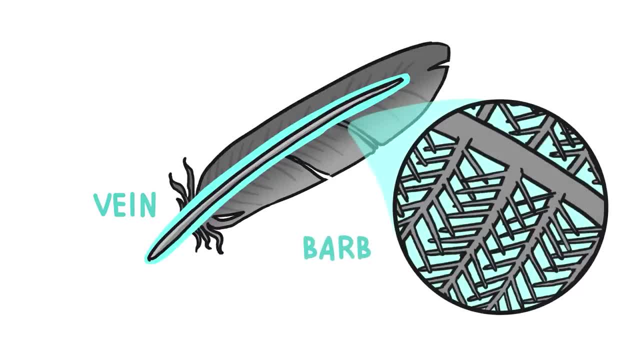 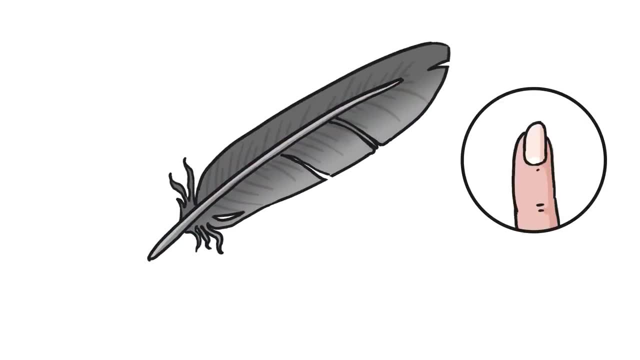 Each feather has a central vein with little hair-like barbs to either side that interlock like little zippers which make the feather act like a little kite. Feathers are made of keratin, which is the same stuff your fingernails are made of. Keratin is great for feather making. 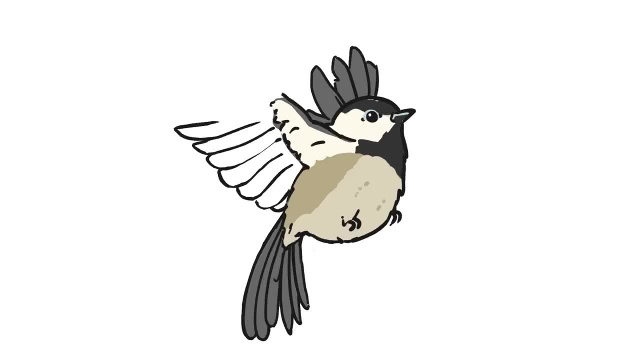 because it's both strong and light. All of the feathers of a wing work together to give the wing as much surface area as possible in order to catch the most air. In order to keep air flowing across those feathered wings, birds need really strong muscles, and even those muscles still need. 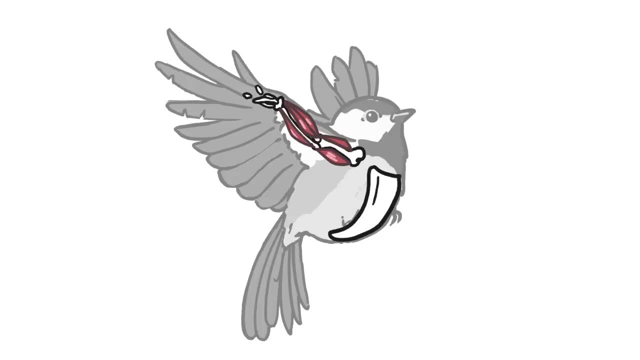 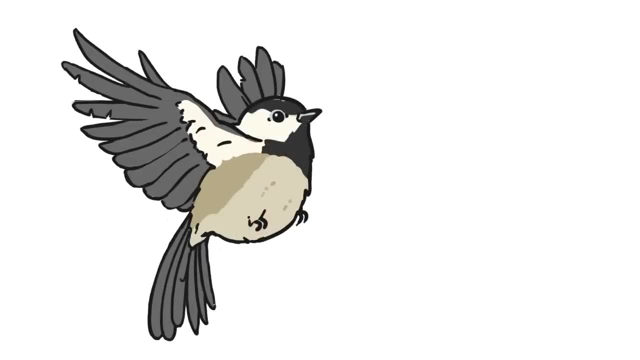 a little help. That's why a bird's wing flapping muscles are anchored to a strong bone called the keel bone, which makes it easier for those muscles to keep flapping the wings. Because flying takes more energy than running, birds have to take in a lot of oxygen to keep from getting out of breath. 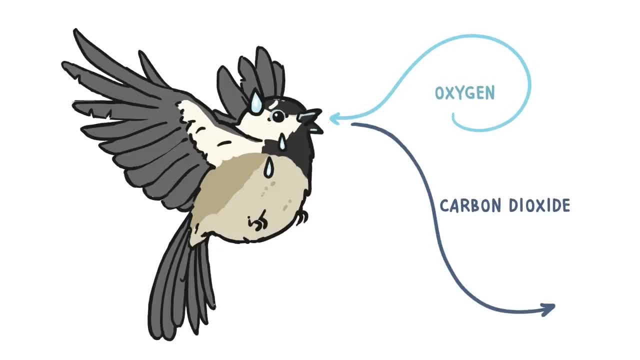 This means that birds have really hard time flapping their wings and they have to be really efficient and kind of weird respiratory systems. They don't just have two lungs like we do. they also have air sacs tucked away in their bodies to hold extra air. Birds also have a. 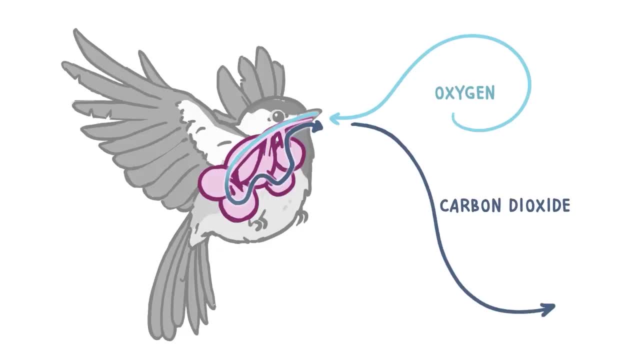 one-way respiratory system. The air takes a linear path from the air sacs to the lungs and back out. In this way, air travels through a bird's body, the way blood travels through your arteries. Speaking of arteries, birds also have really big hearts to pump blood to their energy-hungry. 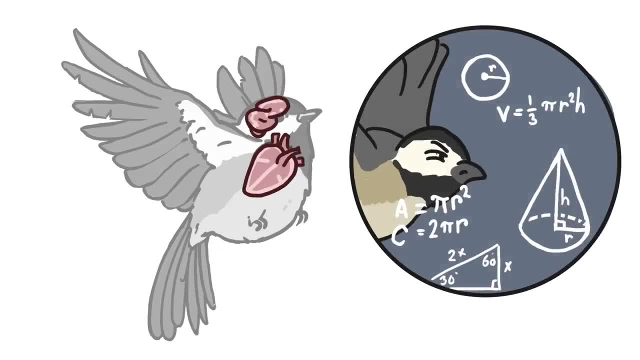 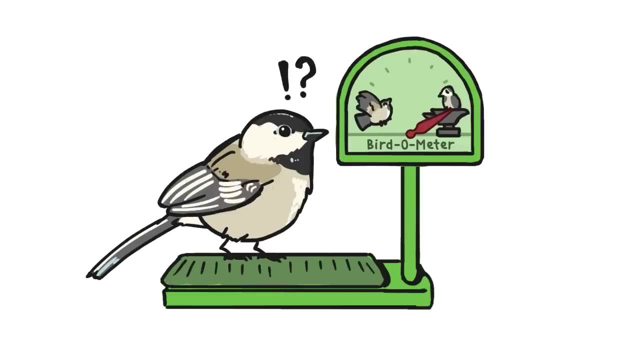 lungs. They also have big brains because flying requires smarts. I mean they have to be quick thinkers to avoid flying into trees. But there is a trade-off: For some parts to become heavier, others had to become lighter. For example, birds lost many unneeded bones like fingers and even. 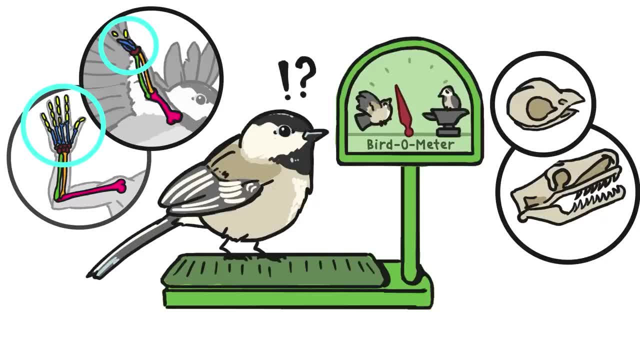 gave up their teeth and jaws, opting instead for lighter beaks. Birds don't even bother with a bladder. In other words, birds can't even hold their pee because it might weigh them down too much. This seems like a lot of trouble to go to just a little bit, But if you're a bird lover, you should. 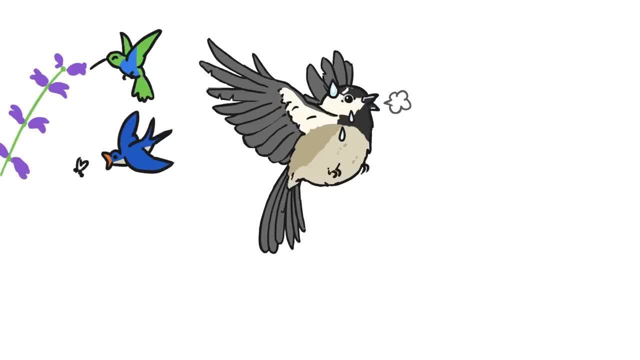 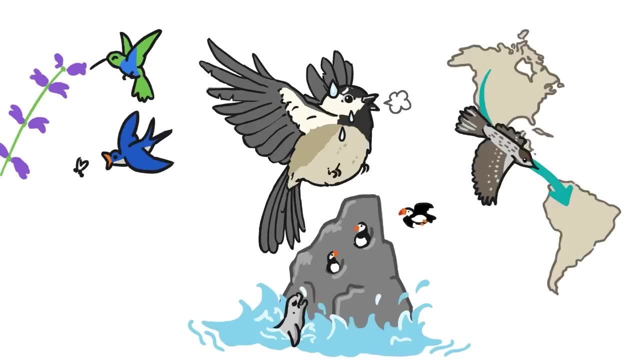 be able to fly. But flying lets birds forage for food in ways that other animals can't, and it allows them to build their homes in places that hungry predators have a hard time getting to, Not to mention birds can travel all over the world. Not even oceans get in their way Flying. 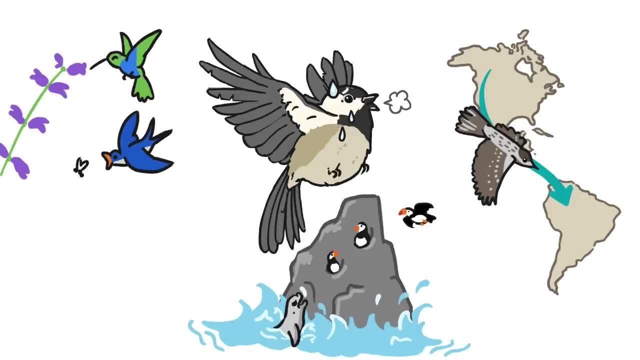 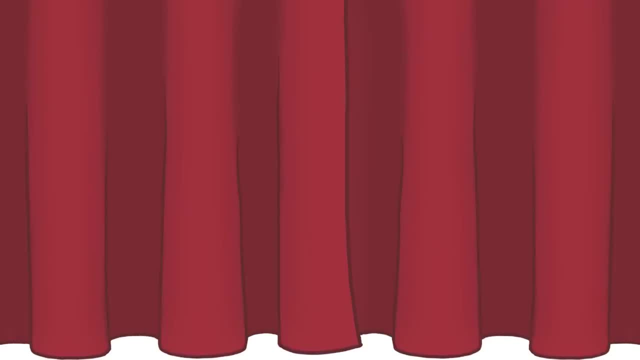 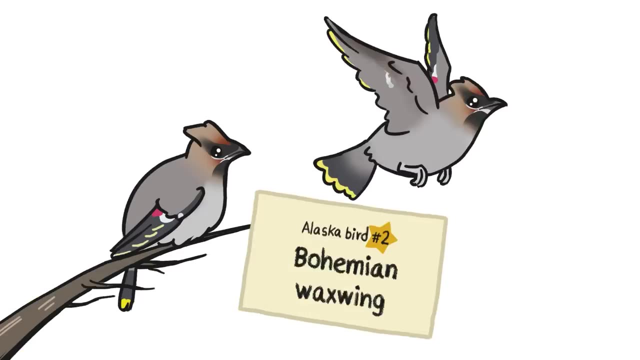 requires lots of adaptations and lots of sacrifices, But if you ask a bird, the best way to get around is to get off the ground. Being able to fly means that birds can move around from place to place pretty easily. Almost half of bird species use their wings to migrate, which means they travel to a different place when the 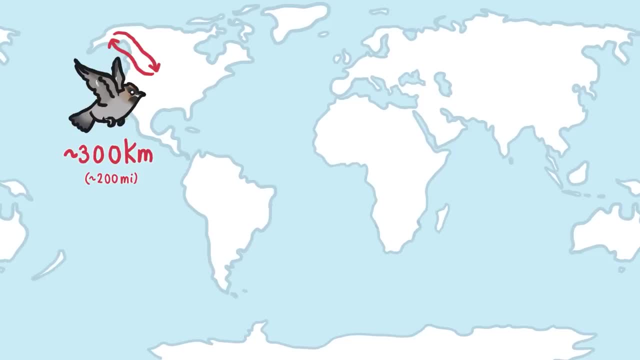 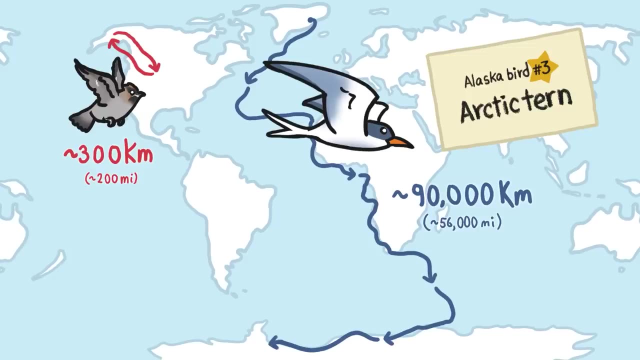 seasons change. Some of them, like the waxwing, only migrate a few hundred miles, while the arctic tern has the longest migration in the world, flying from the farthest reaches of the north to the farthest reaches of the south and back again. every single year, A bar-tailed godwit spends its 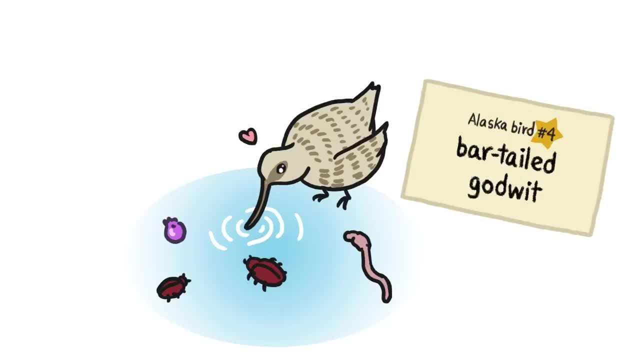 summers in Alaska, where it happily probes for birds. But if you're a bird lover, you should keep in mind that there are a lot of different species of birds in the world and you can't always find them anywhere else in the world. 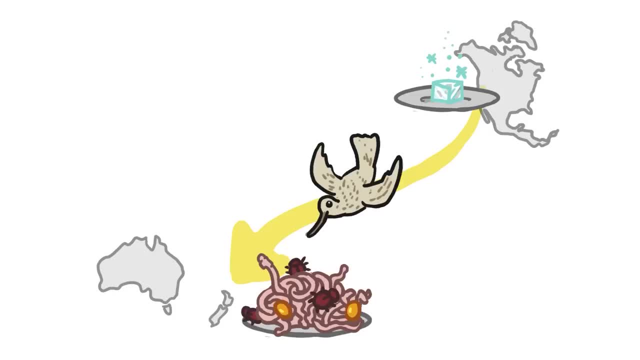 But when summer's bounty ends, most of that food goes away and the godwits fly to warmer climates where food is more abundant. But they can't stay there forever either. Many of these southern spots are crowded with birds, migrants and residents alike, so the godwits take to the 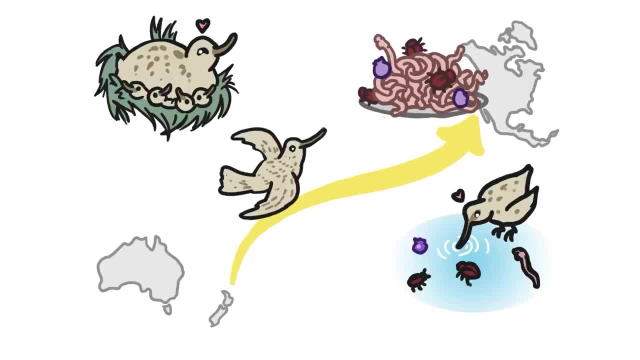 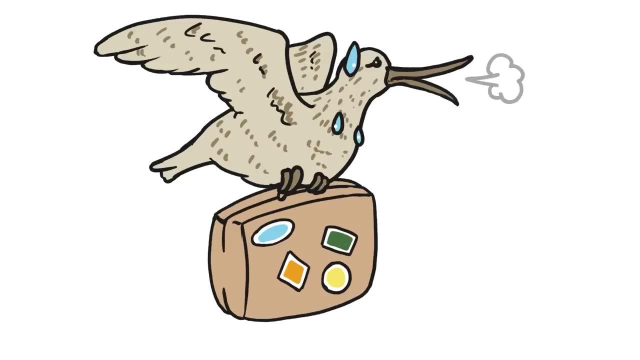 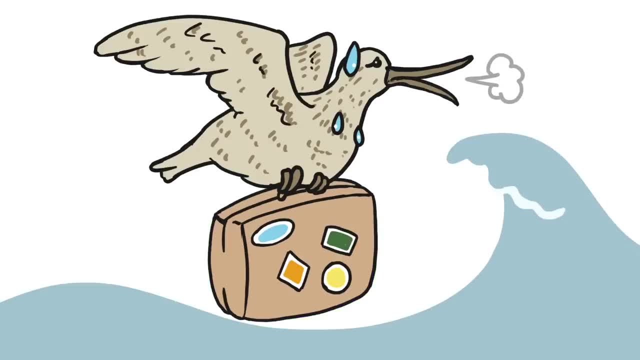 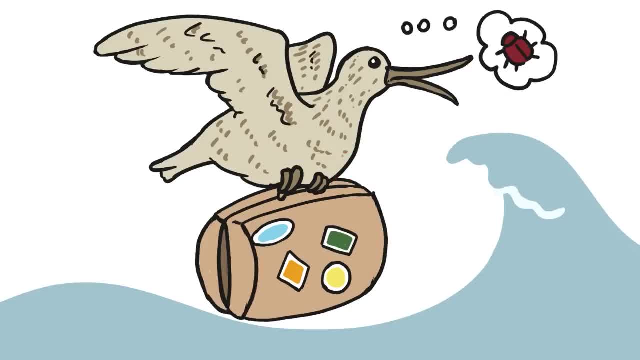 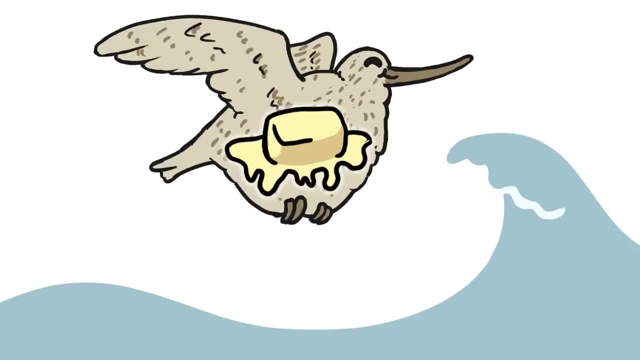 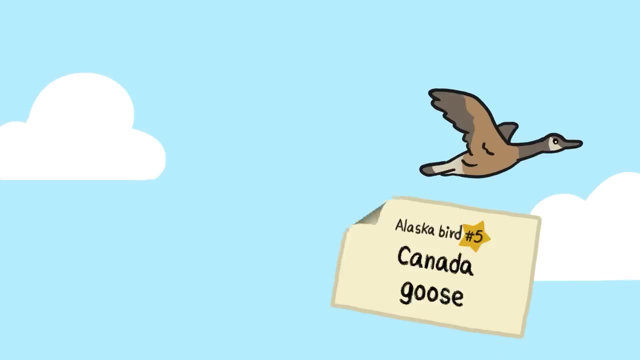 so they take care to pack for their journeys. By pack I mean pack on the fat. When the bar-tailed godwit leaves Alaska for New Zealand, nearly 50% of it's mass is body fat to fuel the journey. Many birds also migrate at night, when most would-be predators are sleeping, Some that fly. 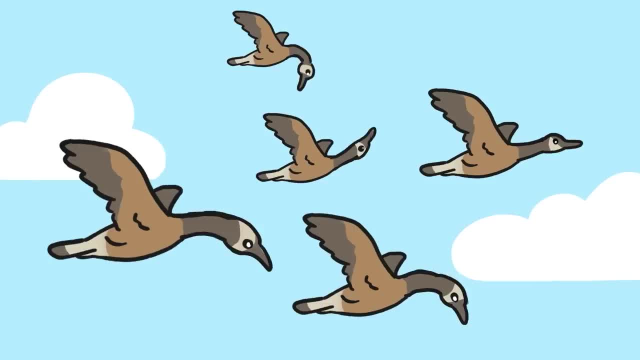 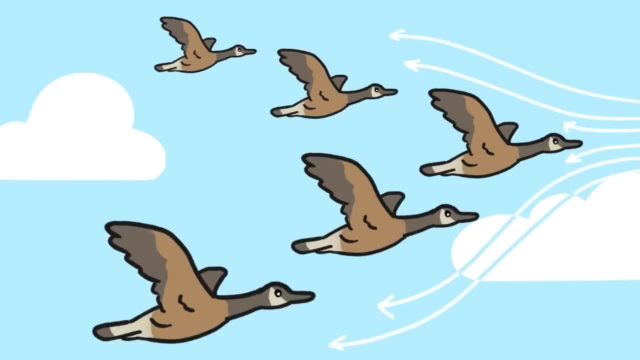 during the day. avoid predators by flying in huge flocks, so more eyes can scan the horizon for threats. Flying in flocks can have an added bonus. Certain formations can reduce wind resistance, which means that each individual bird can spend less energy on the wing. Birds are incredible. 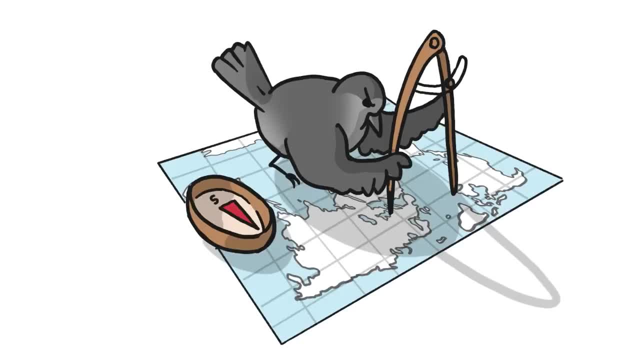 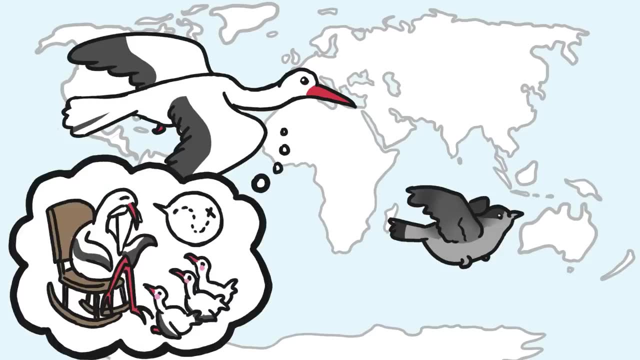 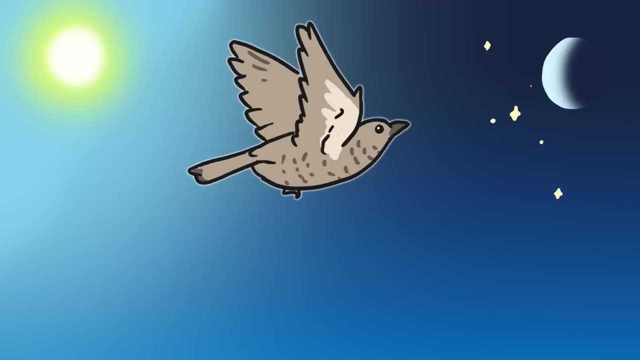 navigators that can travel half the world to find the same patch of forest or ponds every single year. Many birds learn their migration routes from older, more experienced birds, while others make their migrations alone following maps encoded in their genes. They track their positions using the sun, stars and even landmarks like rivers. But when all of 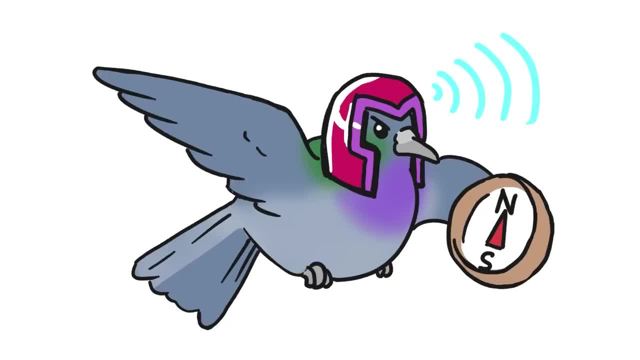 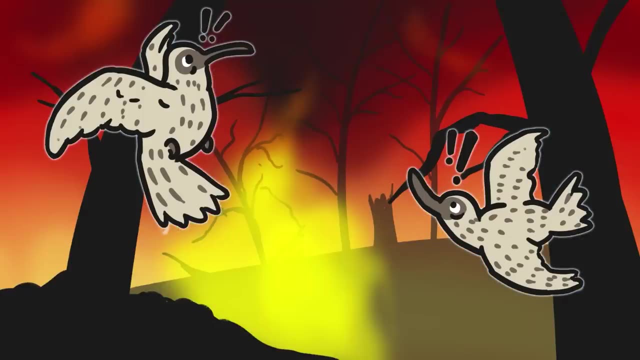 these things fail. some birds can navigate by sensing the Earth's magnetic field, although scientists aren't completely sure how they manage to do it. But birds can't control everything. Hurricanes and other storms make flying over the ocean perilous, while wildfires and floods can destroy stopover habitat. Humans pose a risk to migrants too. Light pollution- 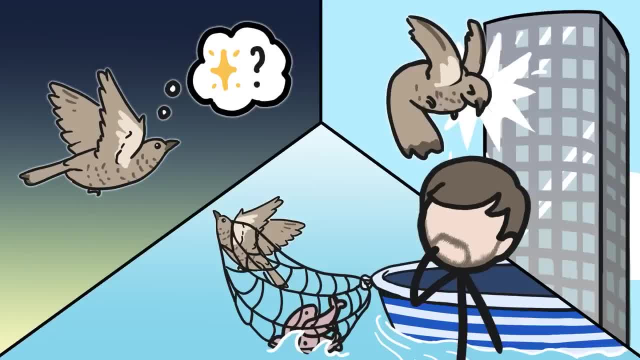 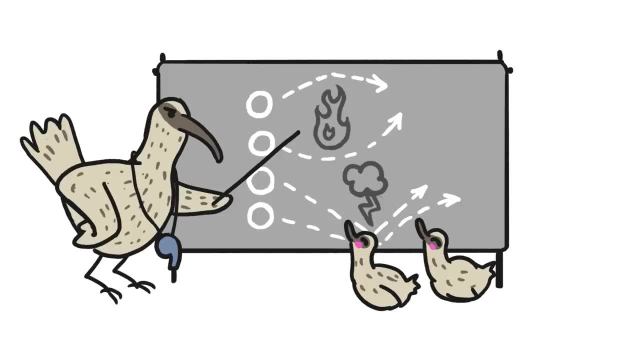 tall buildings and even fishing nets are all dangers that birds face on the surface of the ocean, But they can't control everything. They can't control everything And as the climate continues to change and landscapes continue to shift, birds have had to change their migration strategies. in response, Some are starting. 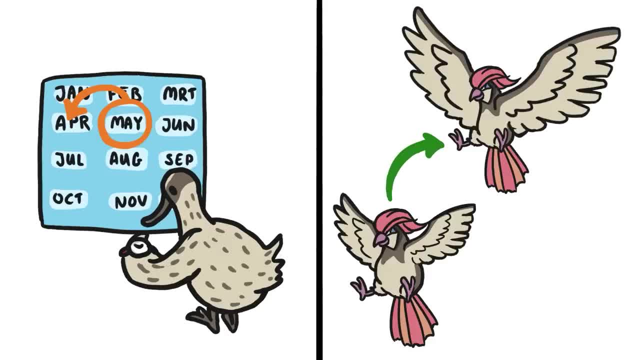 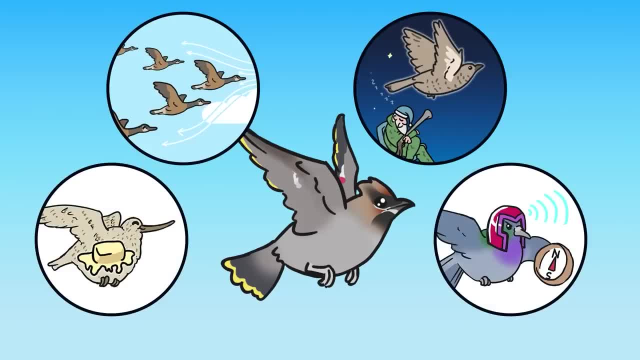 their migrations earlier, while others are shrinking their bodies and lengthening their wings to deal with leaner, more stressful flights. Thanks to skills they've honed over the millennia, migrating birds are adjusting to the new world. They might be flying into the unknown. 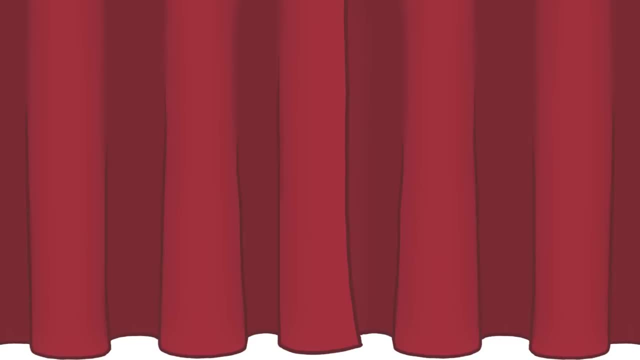 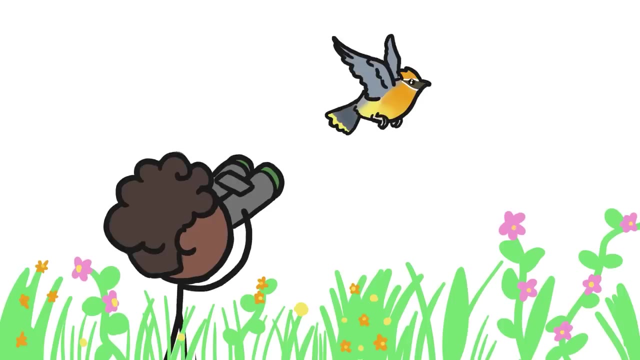 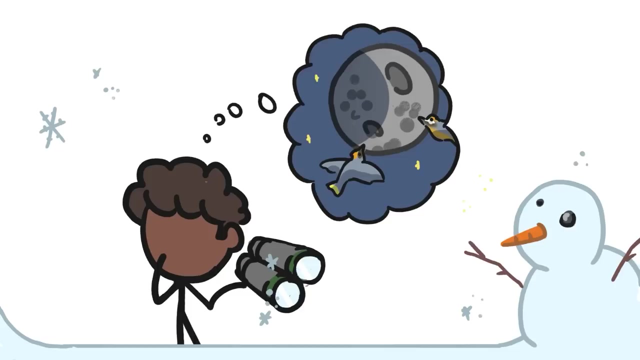 but they aren't totally winging it. Humans have long noticed that birds have a tendency to disappear, at least for part of the year. At first they had no idea where the birds went off to, but that didn't stop them from making some pretty creative guesses. 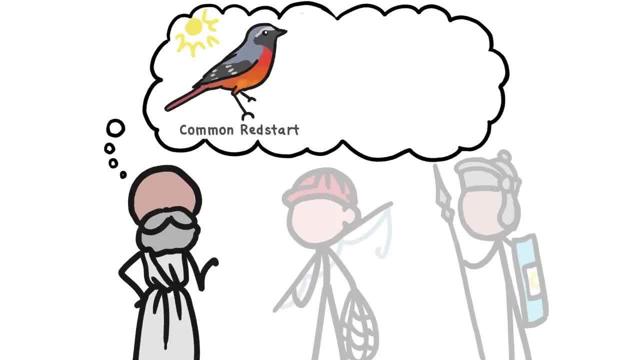 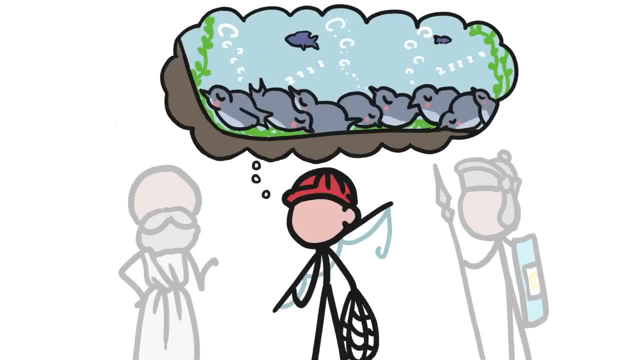 The Greek philosopher Aristotle suggested that redstarts, which spend summers in Greece, annually morphed into robins, which only spend winters in Greece, While later a predominant theory held that some birds hibernate on the bottoms of lakes And people as far back as the 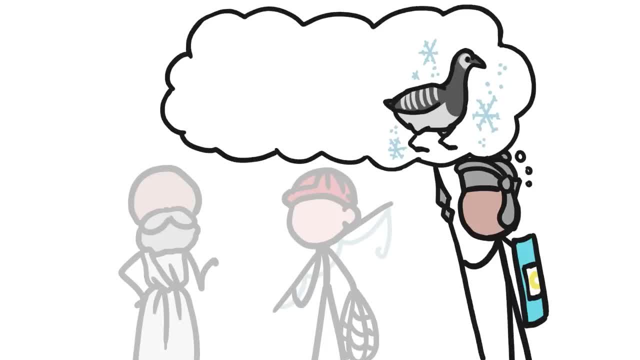 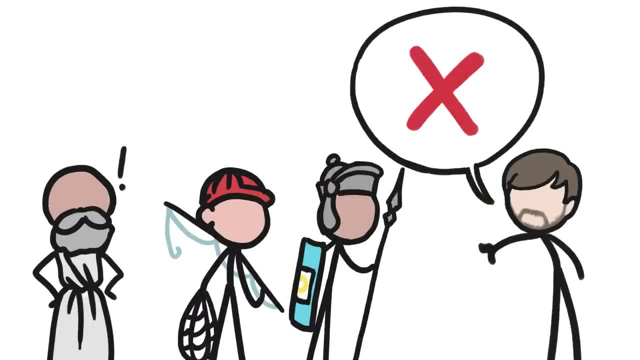 Roman Empire, the Roman Empire and the Roman Empire. the Roman Empire and the Roman Empire assumed the masses of geese that arrived every year were hatching out of barnacles. We now know that they were all wrong. These ideas persisted because, for most people, 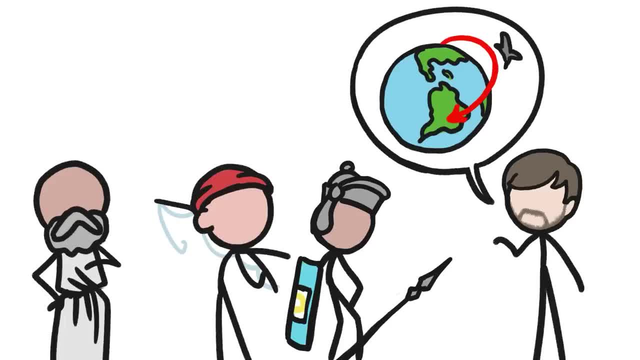 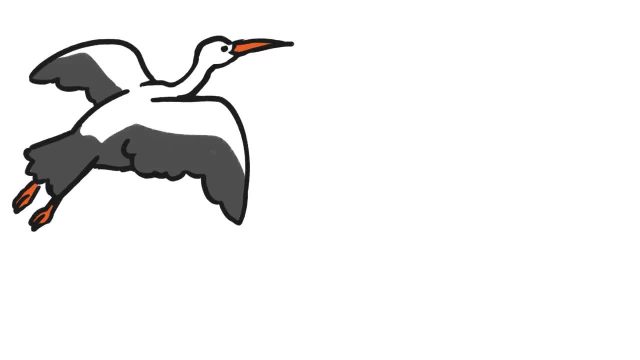 the idea that some birds spend half the year halfway around the world would have sounded even more absurd. One of the first hints that birds spend time abroad came in the form of an accidental message from an African hunter in 1822, when a stork arrived alive in Europe with that. 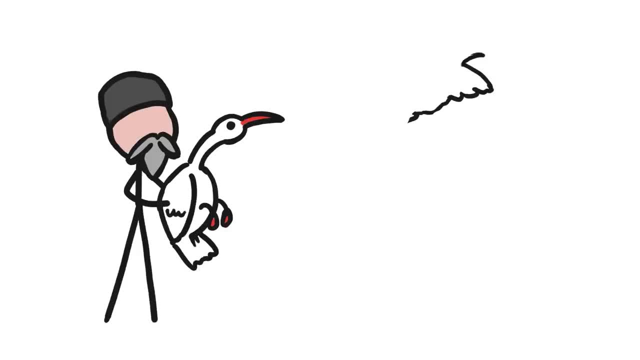 hunter's spear sticking out. This was the first time a stork had ever been seen in the world. This was the first time a stork had ever been seen in the world. Fast forward 80 years to around 1900, when people began purposefully sending birds away. 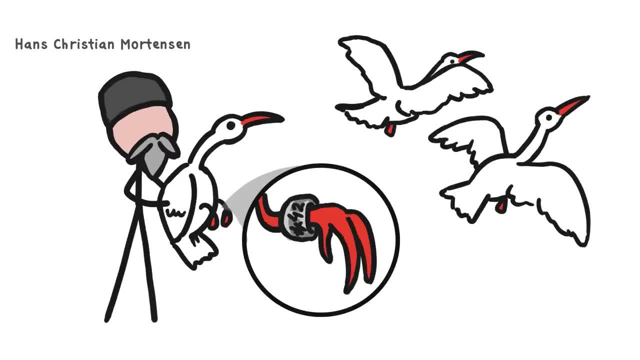 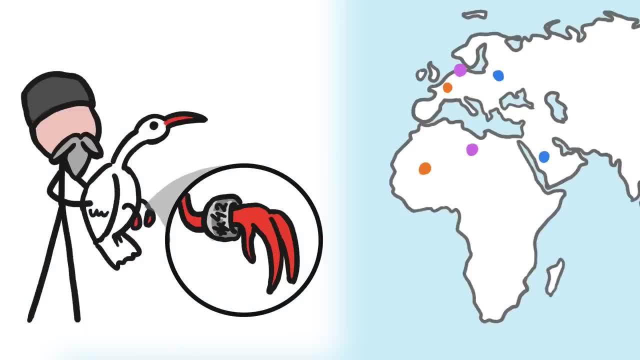 with their own messages. thanks to a Danish teacher's technique of attaching marked aluminum rings to birds' legs and then re-releasing them, Each recapture or sighting of a banded bird put a dot on the map, and soon long-distance migrations were confirmed. when a white stork that had been 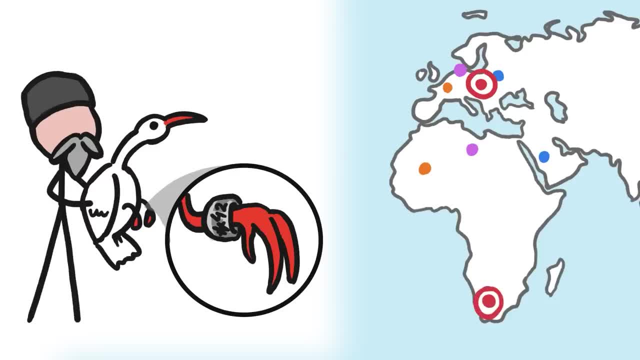 banded in Hungary was found dead in South Africa. But banding can only tell researchers about single points along a bird's migratory path, not what happens between those points. We didn't get our first glimpse of the routes birds took until the 1940s, when it turned out that 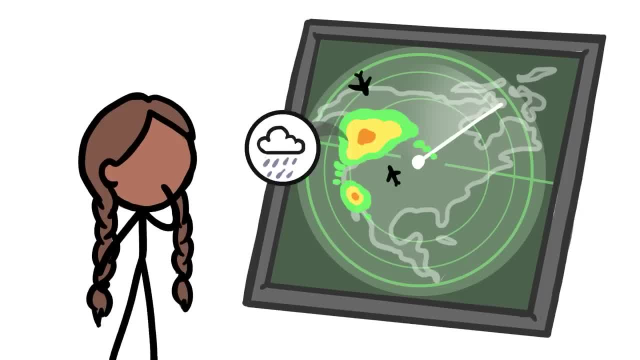 radar, which had been developed to track both airplanes and rain, was also great for tracking masses of birds. Radar allowed us to see the size of migratory flocks moving en masse under the cover of night for the first time. but we weren't able to get individual data until 1984, when a bald 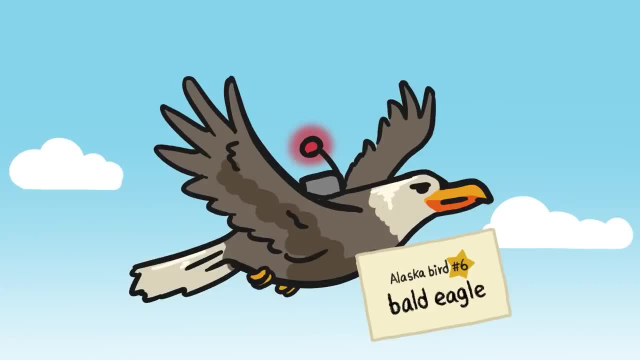 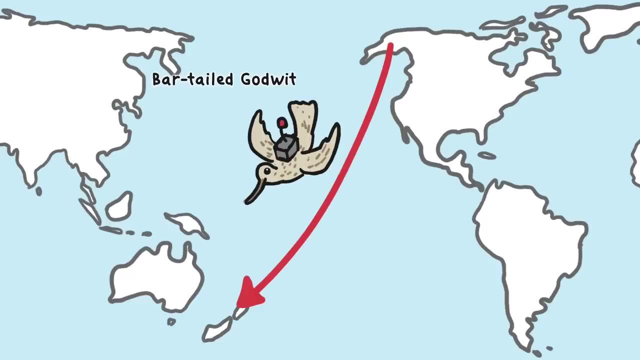 bird was captured and fitted with a transmitter powerful enough to send signals to a pair of orbiting satellites. Satellite tracking revealed details of some remarkable migrations, like the bar-tailed Godwit's annual flight from Alaska to New Zealand, during which the bird covers 11,000. 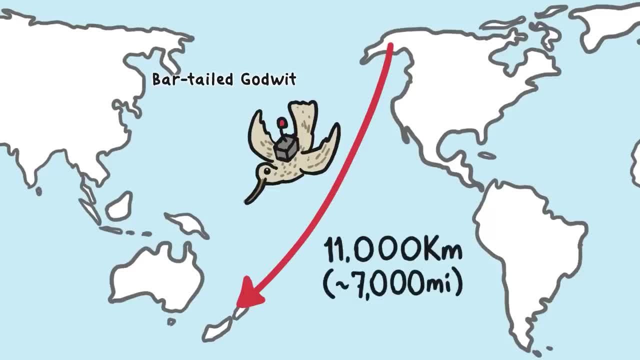 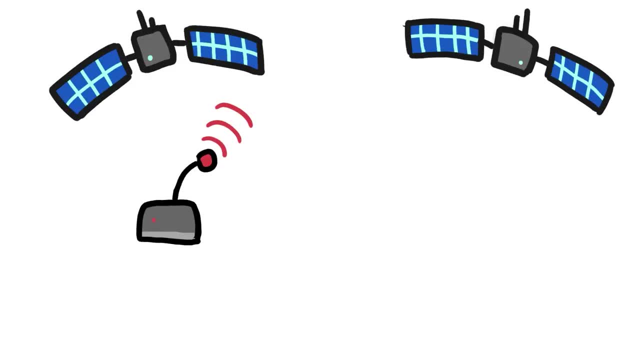 kilometers in about eight days without a single stop. But there's a serious limitation to satellite tracking devices. Even with modern technology transmitters with enough oomph to send signals to satellites are still far too expensive, Even with modern technology transmitters with enough. 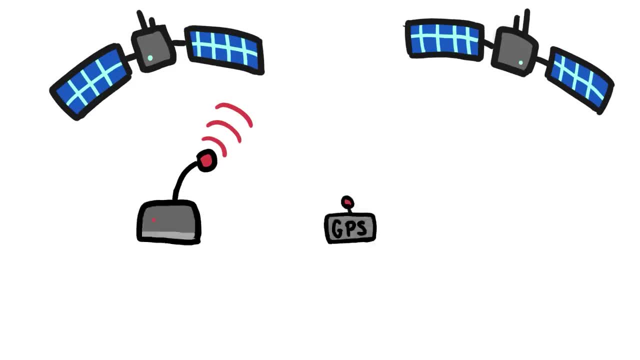 oomph to send signals to satellites are still far too expensive. Even with modern technology, transmitters with enough oomph to send signals to satellites are still far too expensive. A slight improvement is to use GPS recorders, which can be smaller because they receive rather than send. 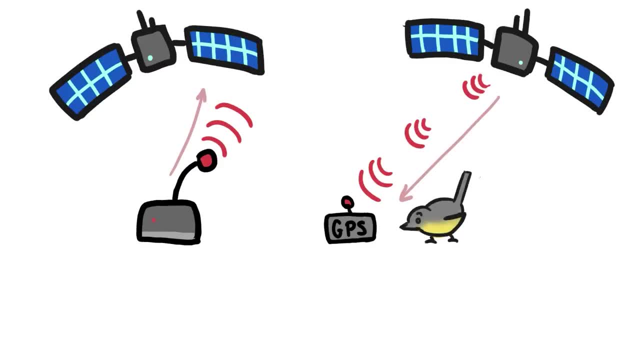 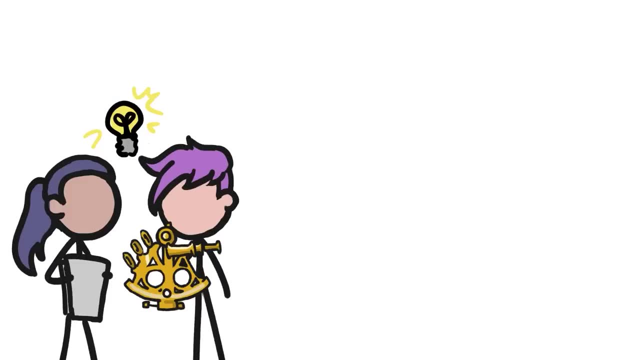 signals to satellites, but they're still far too heavy for the smallest songbirds. Luckily, scientists have been clever enough to realize they don't need satellite tracking at all. Instead, we can fit birds with a tiny device that includes a sunlight detector. 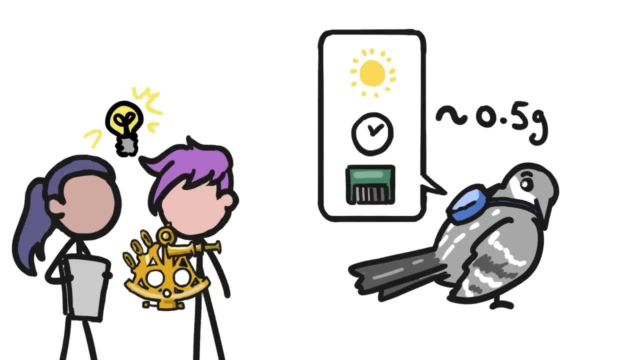 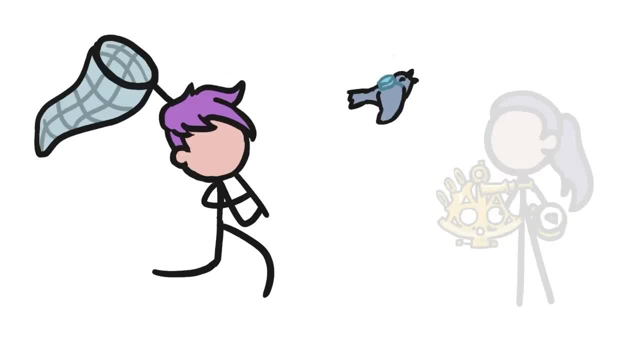 an electronic clock and a memory chip which together weigh as little as a raisin Lightweight light recorders don't broadcast, so we need to recapture the birds to get the data, but we can then use ancient navigation methods to reconstruct the bird's. 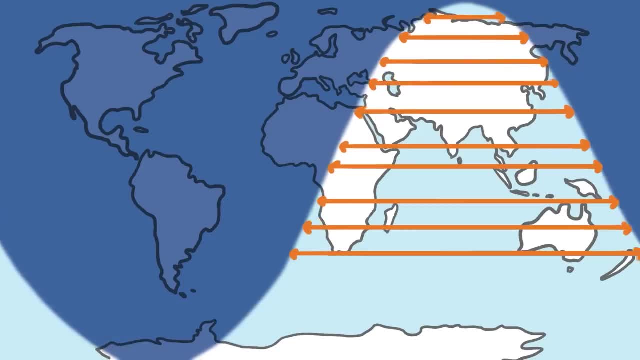 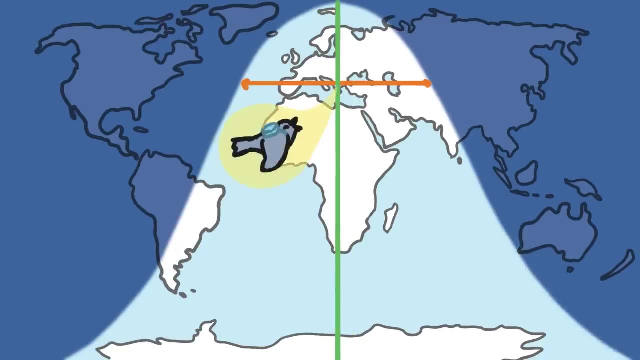 daily location over the course of its journey. The length of each day is an indicator of latitude, and the time halfway between sunrise and sunset, that is, noon, is an indicator of longitude. These clever geolocators have shed light on the world's speediest migration. 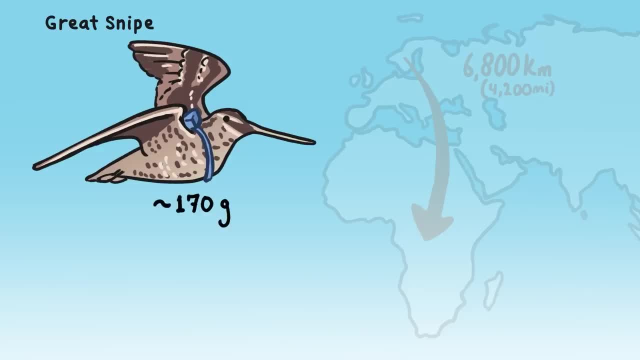 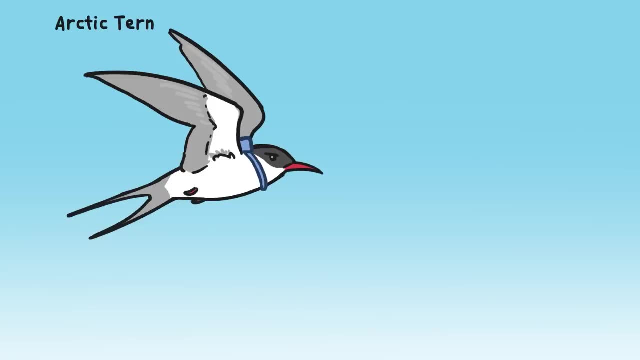 The Great Snipe, which weighs about 170 grams, hightails it from Sweden to Central Africa in just three days, averaging 95 kilometers per hour. Another marathon migrator, the Arctic tern, has long been credited with the longest migration for. 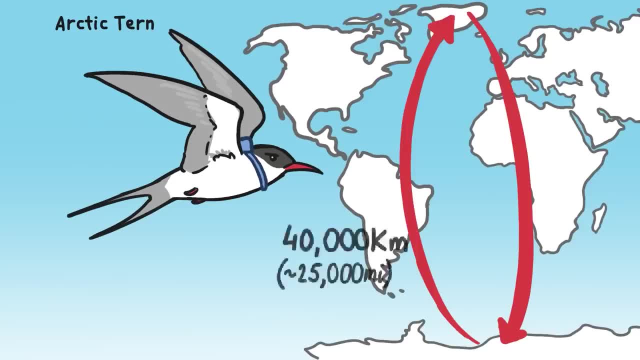 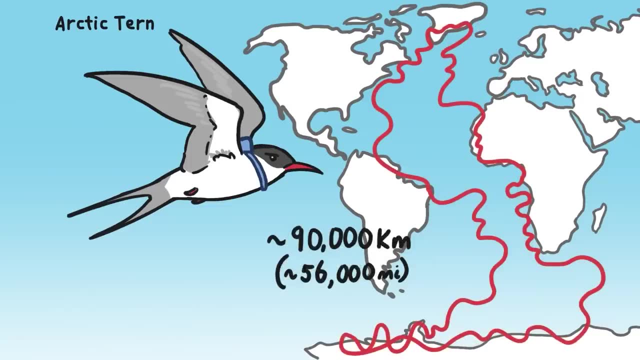 its annual round trip between the Arctic and Antarctic, an estimated 40,000 kilometers, But recent data from lightlevel geolocators show that terns actually travel more than twice as far each year, possibly to take advantage of prevailing winds. While scientists have learned, 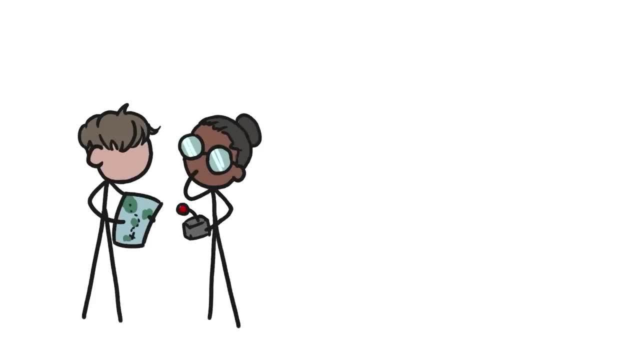 a lot about the specifics of bird migration. they are not the only ones contributing to migratory bird science. Regular folks like you and me are also helping scientists learn about bird migration By pooling the observations of thousands of eager birdwatchers who contribute data to online. 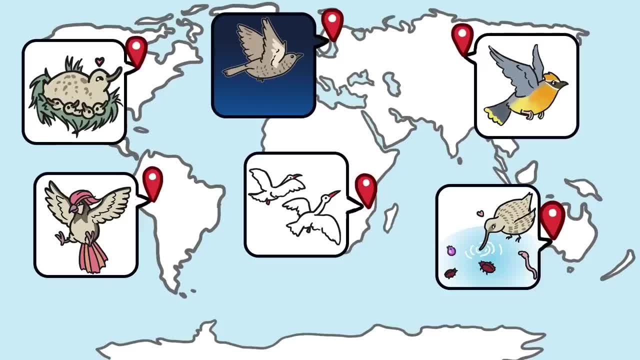 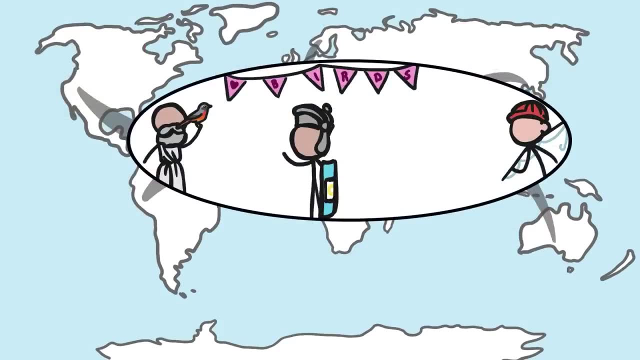 databases, scientists can learn about how migration timings, migratory stopover locations and breeding ranges are changing over time, which would be tough to study with GPS locators alone. So an investigation into migration that began with inquisitive regular folks watching birds is now back to. 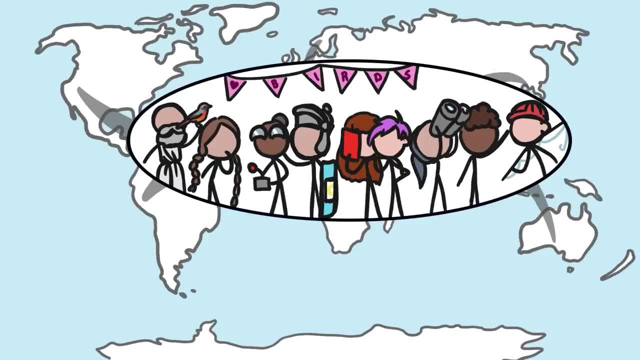 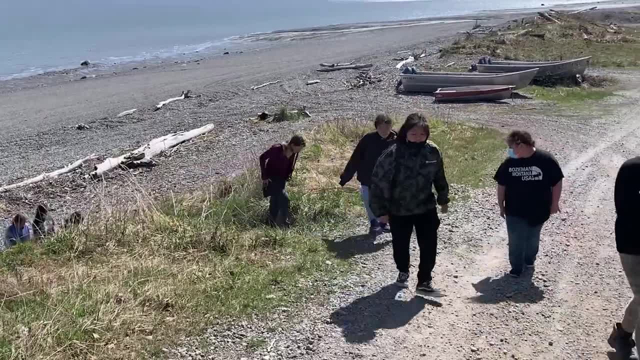 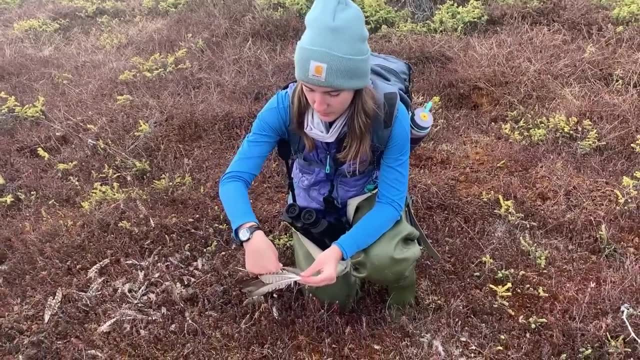 well inquisitive, regular folks watching birds. You might even say we've migrated full circle. We had so much fun working with the students of Tabona School and we are thrilled that we had the opportunity to share their work with you. Remember those bird researchers we mentioned at the start?